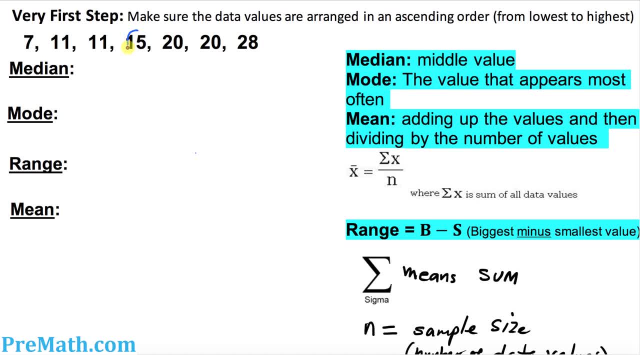 Look at what is the median over here. Of course, obviously 15 is a median number because three values is on the left-hand side and three values on the right-hand side, So median is 15.. So what is the mode? by the way, Mode is simply the number, the values that show up most number of times. 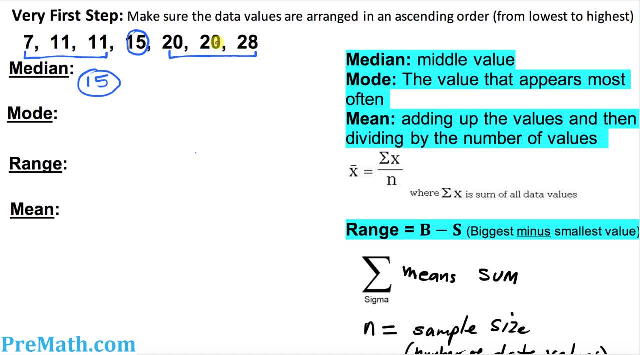 Over here. you can see, 11 is showing up twice and 20 is showing up twice as well. So that means we have two modes. which one are what? 11 and 20 are our modes And they are showing up. how many times They are showing up twice. 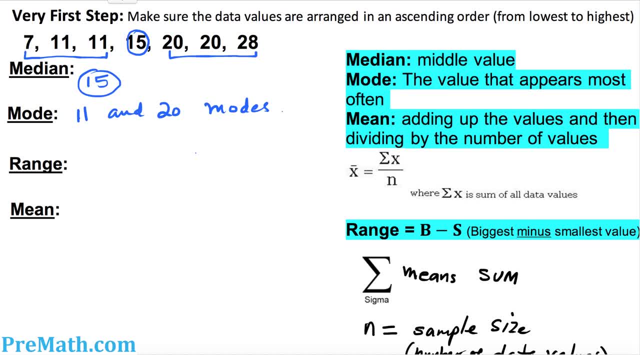 So basically, our range is simply what Range is over here, which look at, the lowest value is what The smallest value is 7 and the highest value, the maximum value, is what 28.. So range is simply what The biggest number minus the smallest number. 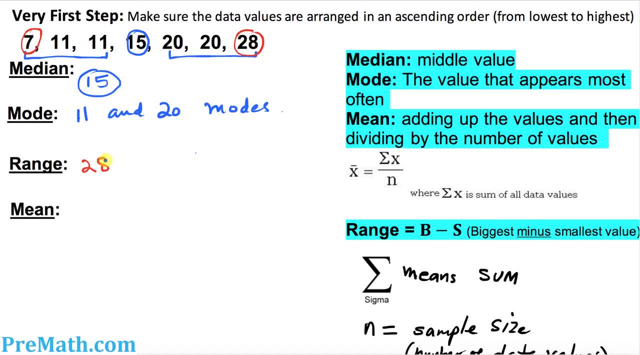 The biggest number is what 28 and minus. you put always a minus and the smallest number is what 7.. And you subtract, So the average is simply that turns out to be 21.. That is our range. And finally, median of, finally mean. I'm talking about mean which is represented by x-bar. 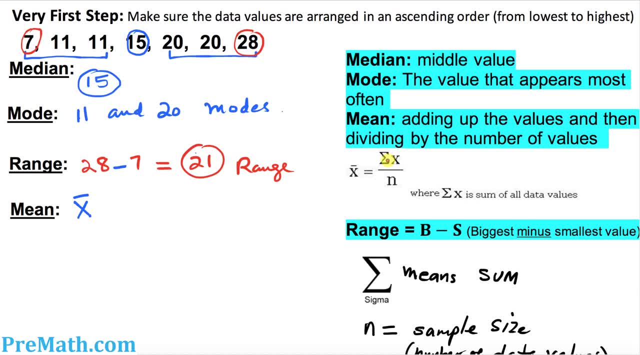 Mean is x-bar. over here, you see, this means that formula is what Sum of the x values? that means all the data values divided by the total number of values. So we wanna add these one up. so this is going to be: x bar is going to be: simply add all these value up, so 7 plus 11 plus. 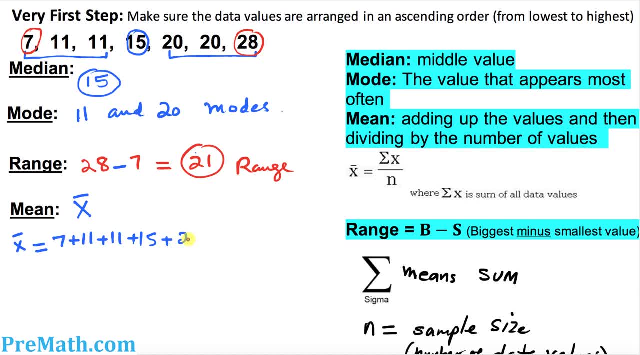 11 plus 15 plus 20 plus 20 plus 28. add them up divided by. look at this thing, how much, how many values are there to data size? are the sample size? is what? 7. so if you add the top part, which is what? 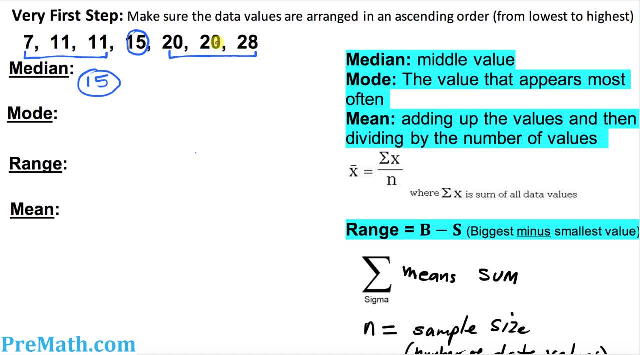 Over here. you can see, 11 is showing up twice and 20 is showing up twice as well. So that means we have two modes. which one are what? 11 and 20 are our modes And they are showing up. how many times They are showing up twice. 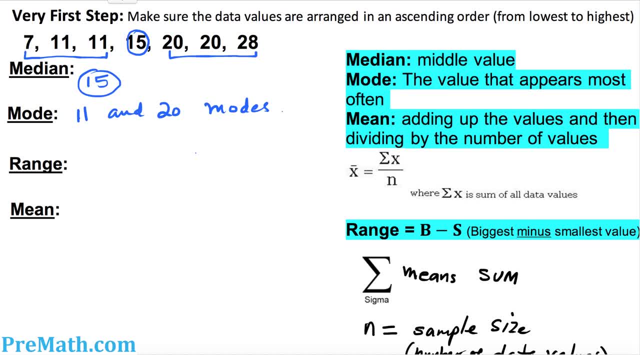 So basically, our range is simply what Range is over here, which look at, the lowest value is what The smallest value is 7 and the highest value, the maximum value, is what 28.. So range is simply what The biggest number minus the smallest number. 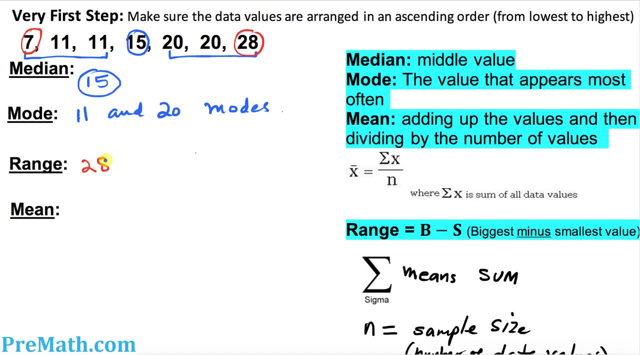 The biggest number is what 28 and minus, you put always a minus and the smallest number is what 7.. And you subtract, So simply that turns out to be 21.. That is our range. And finally, median, finally mean. I am talking about mean, which is represented by X bar. 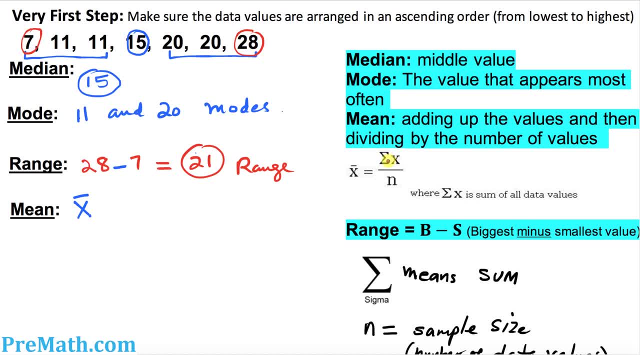 Mean is X bar over. you see, this means the formula is what Sum of the X values? that means all the data values divided by the total number of values. So we want to add one up. so this is going to be: X bar is going to be: simply add all these value. 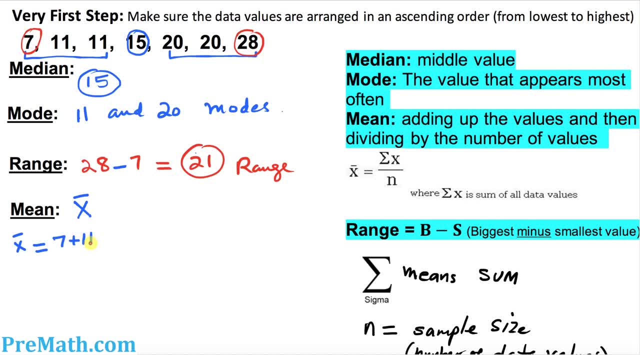 up. so 7 plus 11 plus 11 plus 15 plus 20 plus 20 plus 28, add them up divided by. look at this thing, how much, how many values are there to data size? are the sample size is what? 7? so if you add the top part, which is what? 112 divided by. 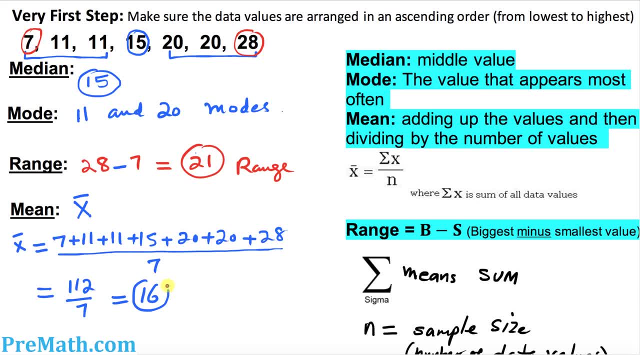 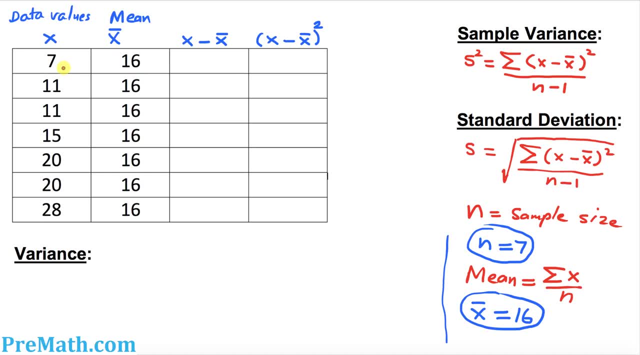 7 is going to give you what 16. so 16 turns out to be our mean. so in this step we will go ahead and fill out all our data values, which we call X values in this table. as you can see, these one, the very first column on the left-hand side. 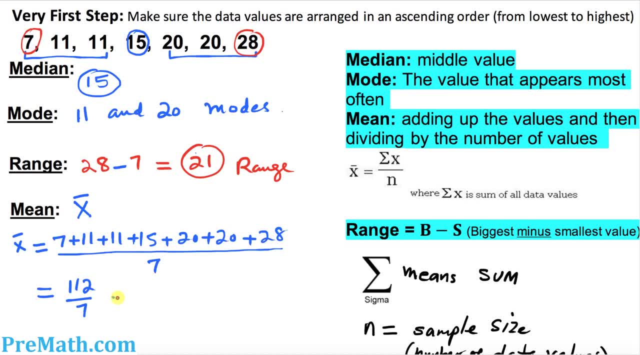 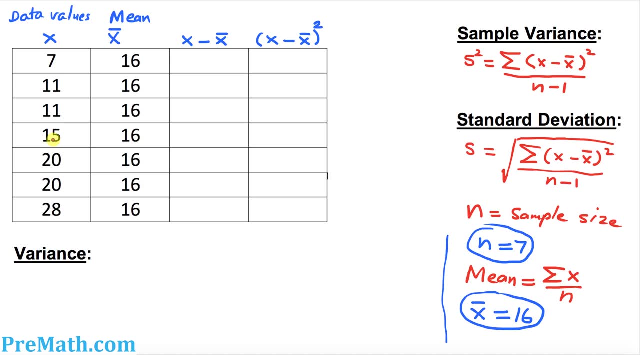 112 divided by 7 is going to give you what 16. so 16 turns out to be our mean. so in this step, we will go ahead and fill out all our data values, which we call x values in this table, as you can see here. so we are going to add all these values to this table and we are going to add all these. 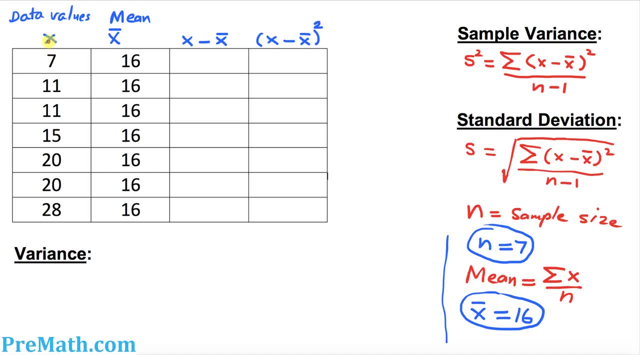 values to this table. as you can see, these one, the very first column on the left hand side, i put down all data values from 7 all the way to 28 and i'm going to call them x values. the next column: i put down all our mean values, which is we call it x bar. we figured out these values in the previous. 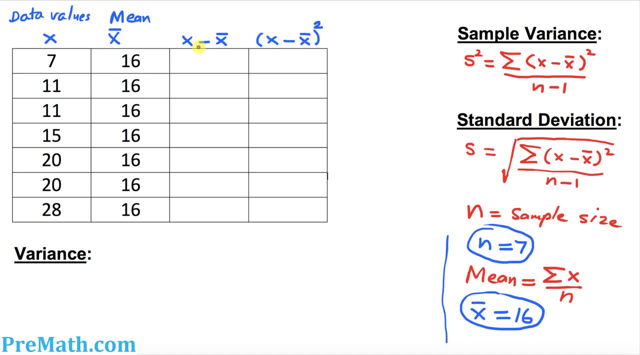 step, as you can see, these one. so the next step, i want you to find: x minus x. bar means x, the first column minus the second column. 7 minus 16 is what negative 9. likewise, 11 minus 16 is going to be negative. 5, 11 minus 16 is again. 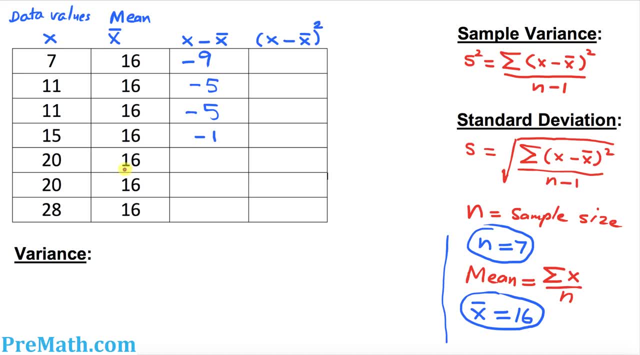 negative 5 and that's going to turns out to be negative 1. this is 4. this is 4. this is what 12. see how we got it: we just simply subtracted these two values and the final column, the right hand side. what we're going to do is: 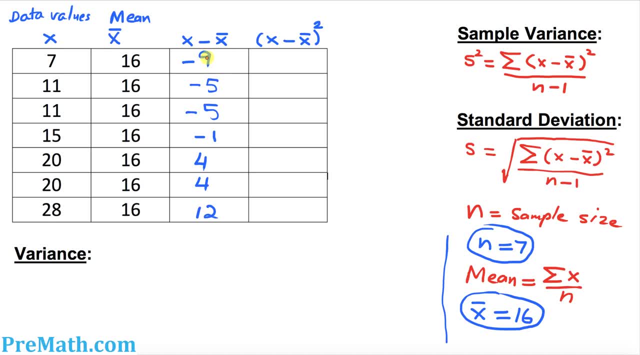 we're going to square the values that we just figured out. so negative 9 squared, negative 5 squared all the way. so this negative 9 squared becomes 81. so negative 5 squared becomes 25, 25, 1, 16, 16 and 144. that's the very first step. we did this one. now what we're going to do is we're going. 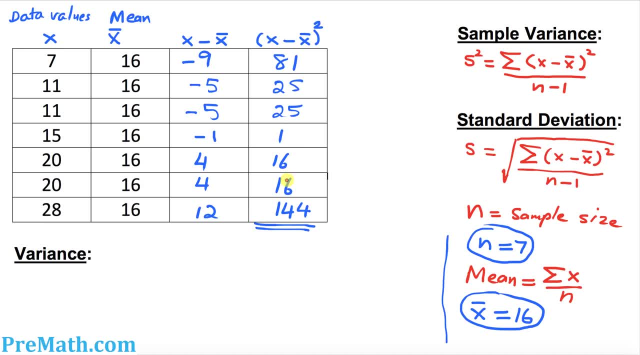 to add these numbers up under this last column, and this is we will call summation sigma notation of x minus x, bar squared. that means we are adding up all these. Sigma means simply add them up. so once we add these things up, this turns out to be what? 3 0, 8. and now we want to find the variance. variance is always repeating. 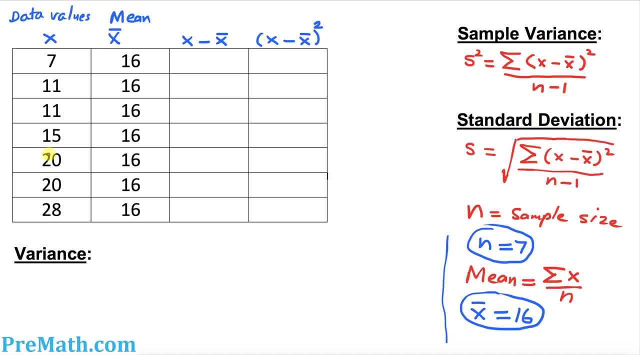 of the table and then we will go ahead and fill out all our data values, which we call X values in this table. as you can see, these one, the very first column on the left-hand side of, I put down all data values from 7 all the way to 28, and I'm gonna call them X. 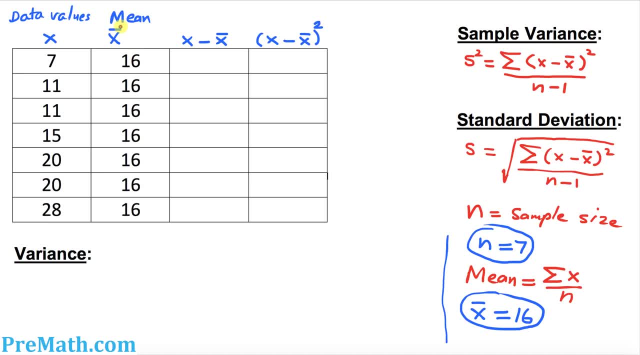 values, the next column. I put down all our mean values, which is we call it X bar. we figured out these values in the previous step, as you can see these one, so the next step I want you to find X minus X bar means X, the first column. 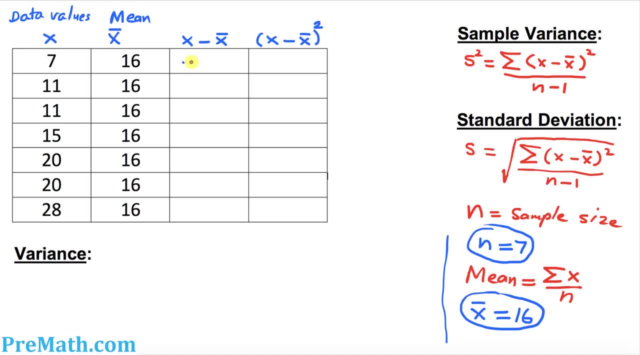 minus the second column, 7 minus 16 is what negative 9. likewise, 11 minus 16 is gonna be negative 5. 11 minus 16 is again negative 5, and that's gonna turns out to be negative one. this is for this is for. this is what 12. see how we got it. 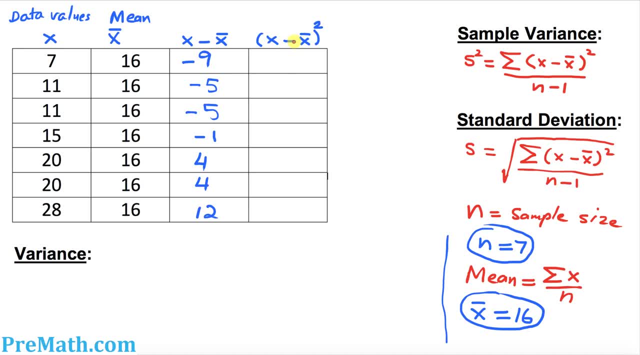 just simply subtracted these two values and the final column, the right-hand side. but we're going to do is we're gonna square the values that we just figured out. so we know this is 15 and 18. we're going on and I'm going to take the topnament now�. 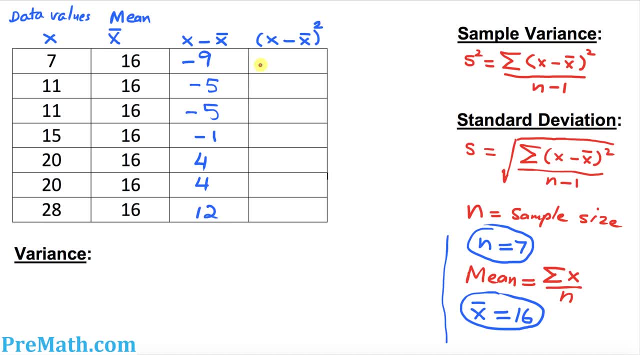 and will take down the bottom element now�. negative 9 squared, negative 5 squared all the way. so this negative 9 squared becomes 81. so negative 5 squared becomes 25, 25, 1, 16, 16 and 144. that's the very 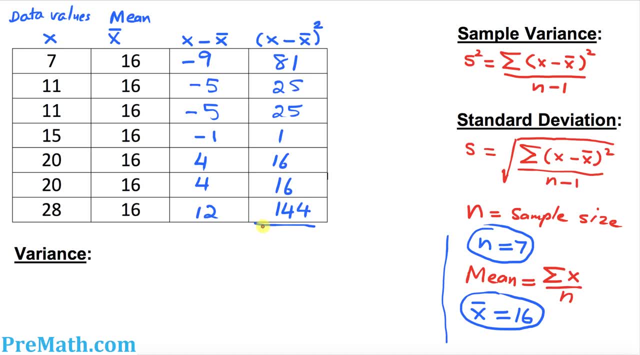 first step, we did this one. now what we're gonna do is we're gonna add these numbers up under this last column, and this is we will call summation: sigma notation of X minus X bar squared. that means we are adding up all the Sigma means, simply add them up. so once we add these things up, this turns out to be a. 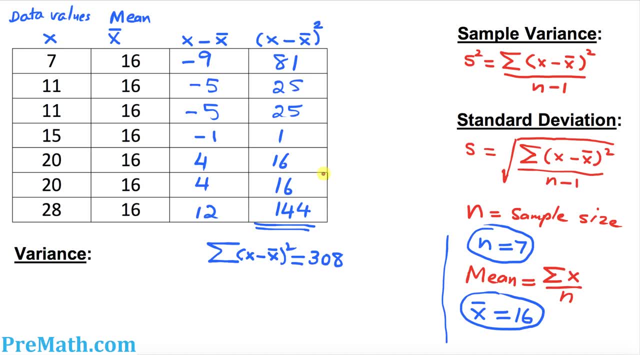 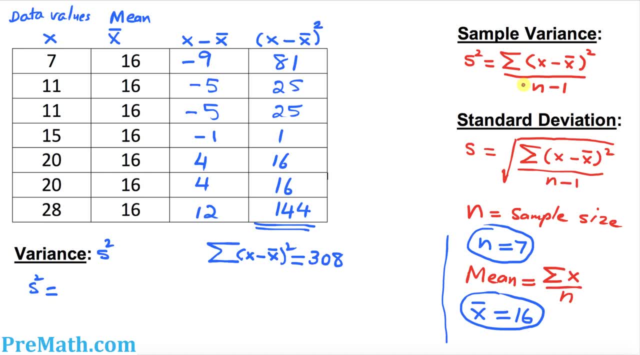 squared. the formula is on the right hand side, as you can see. this is what X minus X bar squared divided by N minus 1. so we figured out this one right up here, which is 3 0, 8 divided by n is how much we. 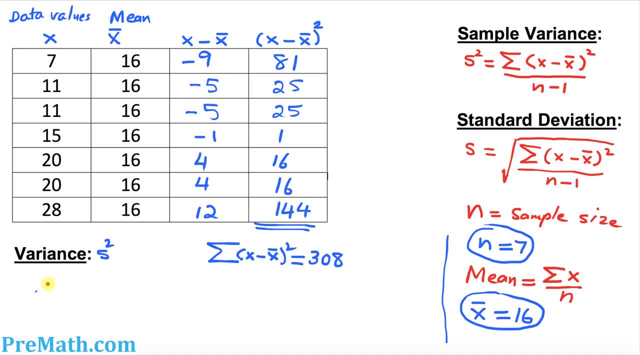 represented by s square, so our variance is going to be simply s square. the formula is on the right hand side, as you can see. this is what x minus x bar square divided by n minus 1. so we figured out. this one right up here, which is 308 divided by n, is how much we know that these data values, these 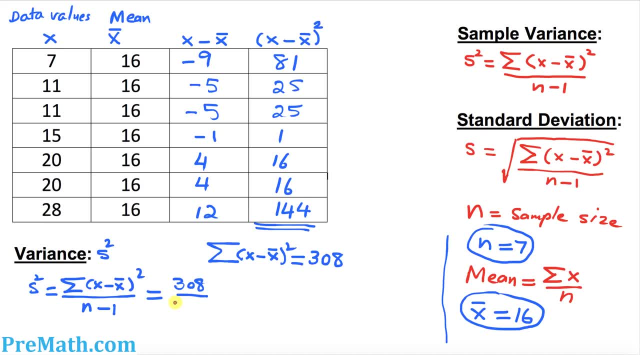 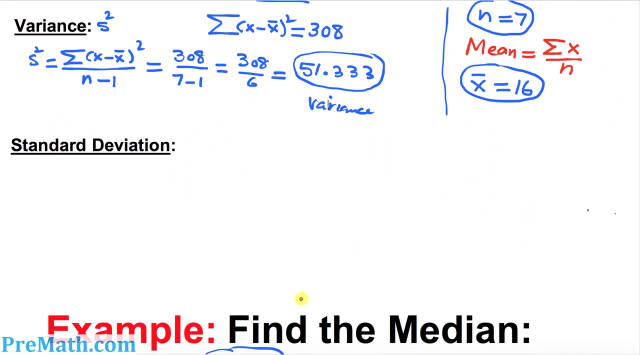 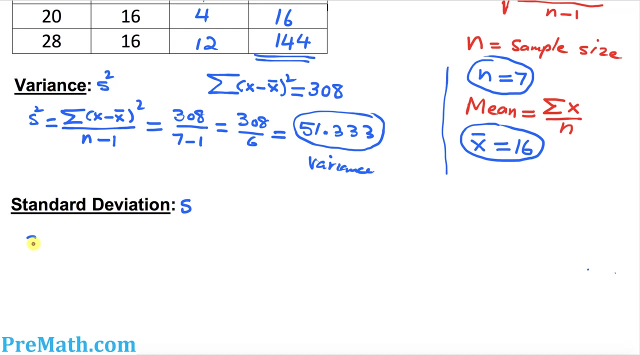 these values are seven of them. seven minus one becomes six, of course. 308 divided by six is going to give you 51.333. goes on and on and on. this is our variance, and now we're going to figure out the standard deviation. standard deviation is always represented by s. so simply, s is going to be simply. 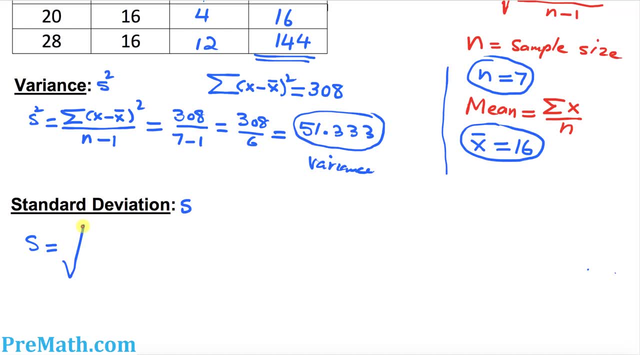 what the formula is this thing? the square root of sigma x minus x, bar squared divided by n minus 1. so we know that this on the top is 308 divided by 6. that is what square root of 51.333 if you take the square root of this. 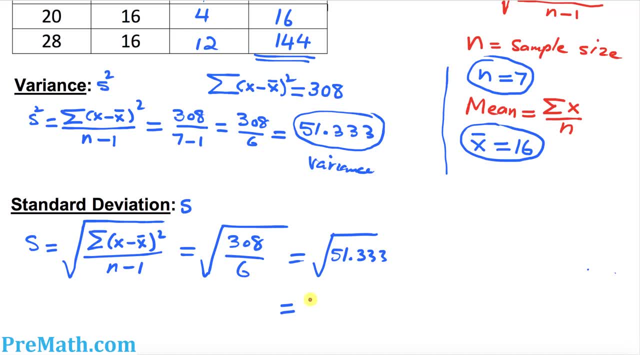 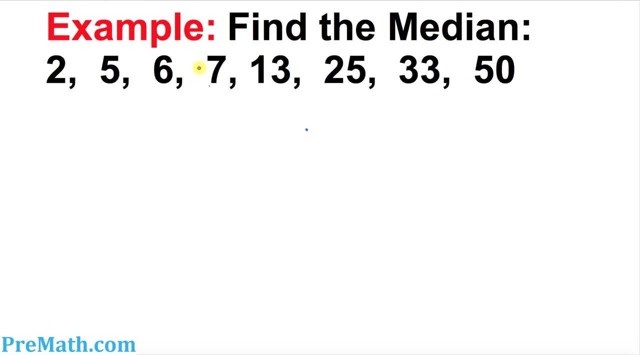 one. that is going to be how much? seven point one, seven point one, six five is our value. so thus our s turns out to be a seven point one, six five. that is our answer. and finally, in this example over here, we've been asked to find the median. so what is going to be the median in this? 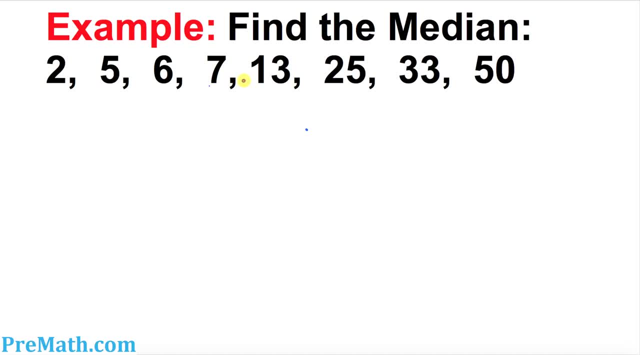 one over here. if you look at the median median is. median is going to be somewhere in the middle. median means what? the middle number? we know that thing. so the middle number is going to be right in between. so right now over here, how we find, when we have a two numbers and we want to find the middle number, we just 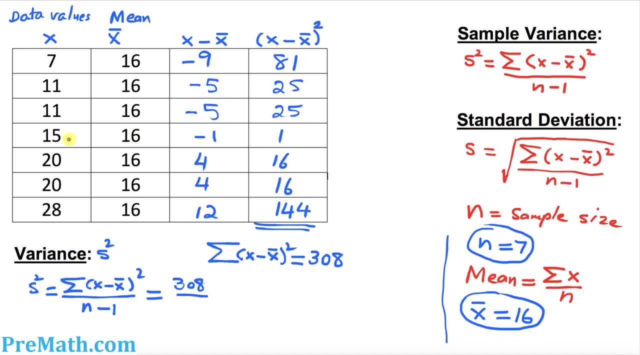 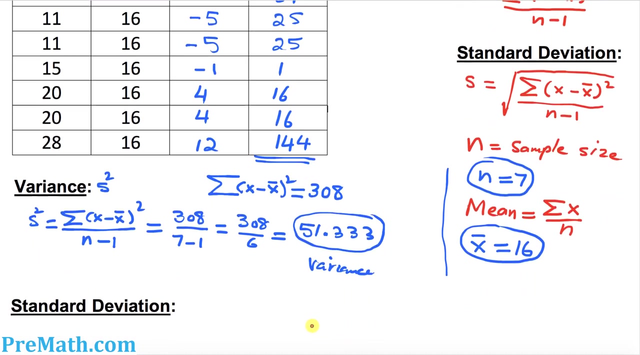 know that these data values, these, these values are seven of them. seven minus one becomes six, of course. three, zero, eight divided by six is gonna give you fifty. one point: three, three, three goes on and on and on. this is our variance, and now we're going to figure out the standard deviation. standard deviation is always. 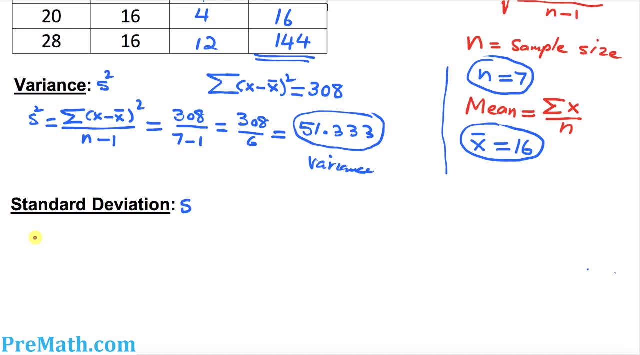 represented by s. so simply s is going to be simply what the formula is this thing: the square root of sigma X minus X, bar square divided by n minus 1, so we know that on the top is 308 divided by 6. that is what square root of 51.333, if you. 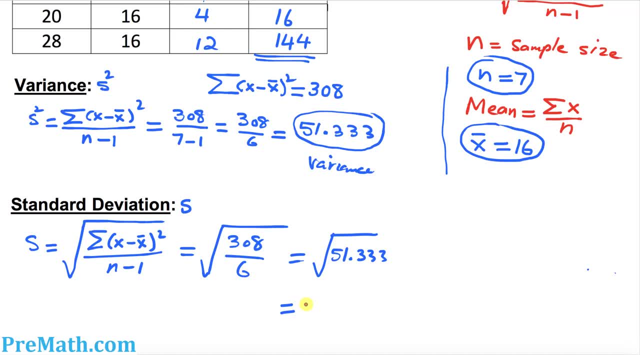 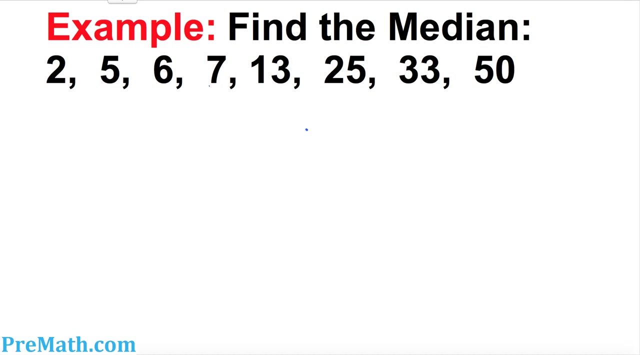 take the square root of this one, that is going to be how much? 7.1, 7.165 is our value. so thus our s turns out to be a seven point one, six, five. that is our answer. and finally, in this example over here, we've been asked to find the median. 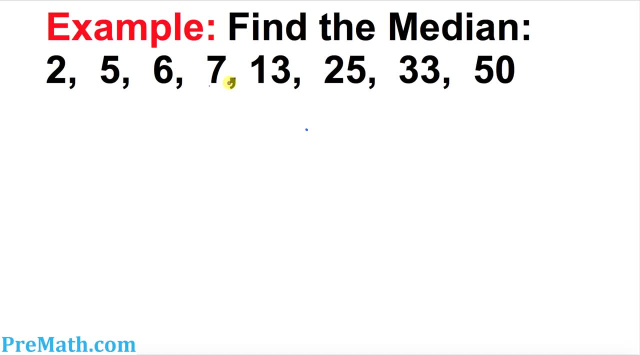 so what is going to be the median in this one over here? if you look at the median, median is median is going to be somewhere in the middle. median means what median is going to be somewhere in the middle, the middle number. we know that thing. so the middle number is going to be right. 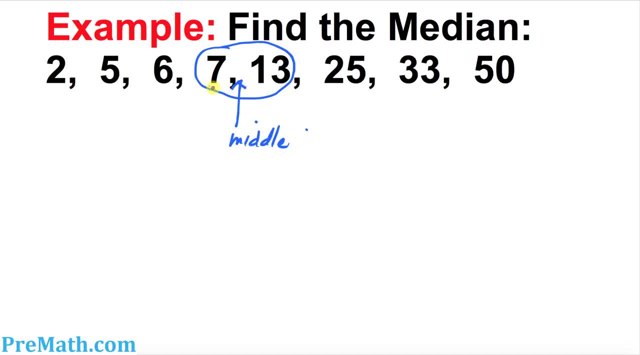 in between. so right now, over here, how we find, when we have a two numbers and we want to find the middle number, we just simply find the average of these two numbers. so median is simply what is? you add these number up seven plus thirteen, and always divided by two, that turns out to twenty over two. so our median is: 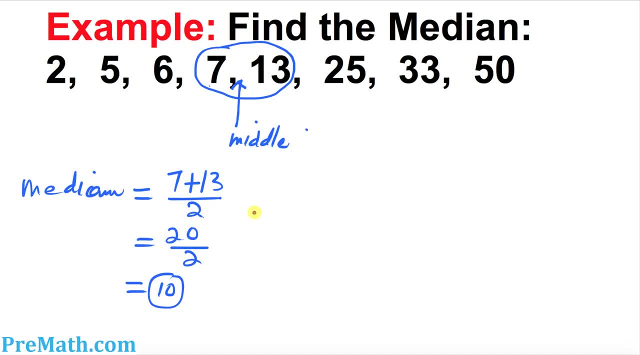 going to be simply ten, and that's our answer. thanks for watching.